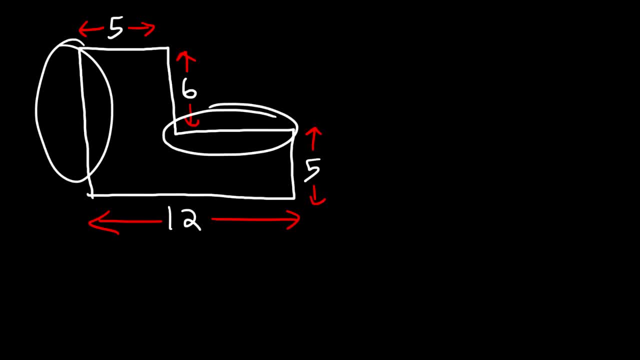 the length of this side and this side. So, starting with the left side, notice that it's simply 6 plus 5 or 11.. So that's 11 units long. Now let's find the length of this side. So notice that we have 12. 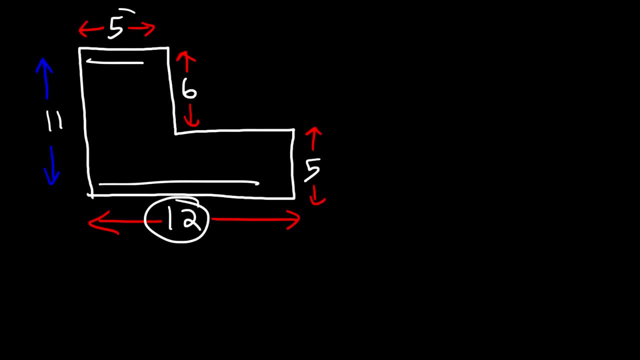 for the entire side, and then this section is 5.. 5 plus some number must add up to 12.. To find that number, it's just 12 minus 5. so therefore this section has to be 7. so now that we know it's 7, we could. 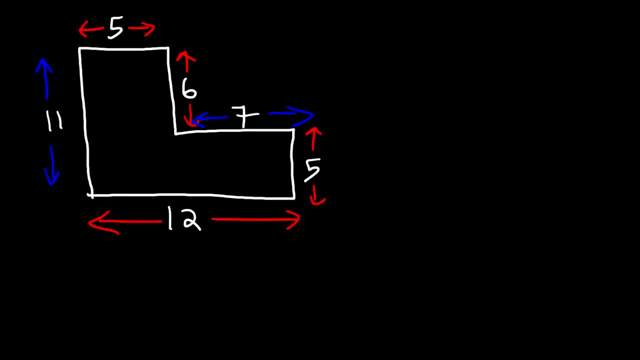 find the perimeter, we just have to add up all the numbers. so it's going to be 5 plus 6, which is 11 plus 7, that's 18. 18 plus 12 is 30, 30 plus 11, that's 41 plus. 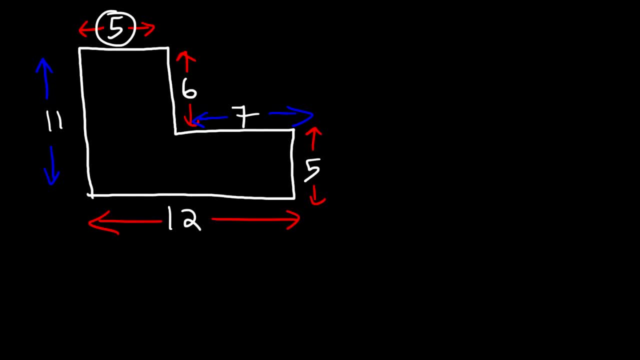 5 is 46, so therefore the perimeter of this figure is 46 units. now let's find the area of this figure. so let's turn this into two rectangles. so the area of this rectangle is simply left times, with 5 times 6, so it's 30 square units. 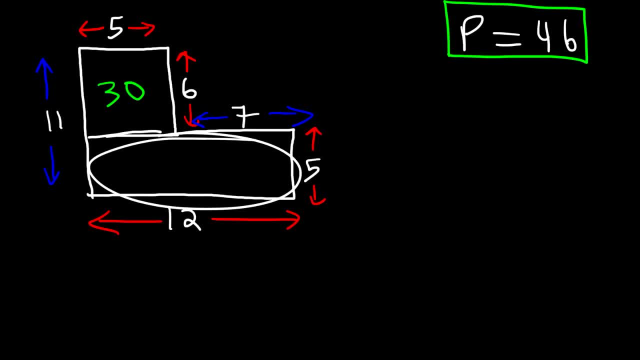 now the area of the second rectangle is also left times with. so it's 5 times 12, which is 60. now to find the total area, we need to add up 30 plus 60, and 30 plus 60 is 90. so that's the area of this figure. now let's work on another example. 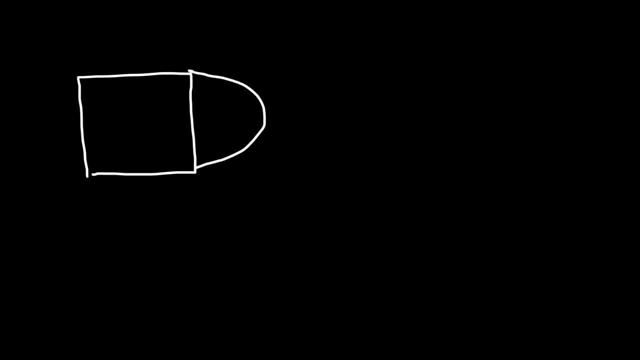 now let's work on another example. so let's say: actually let me draw a different figure. let's say we have a rectangle attached to a semicircle and it measures 5 inches by 6 inches. find the area and the perimeter of this figure. so let's start. 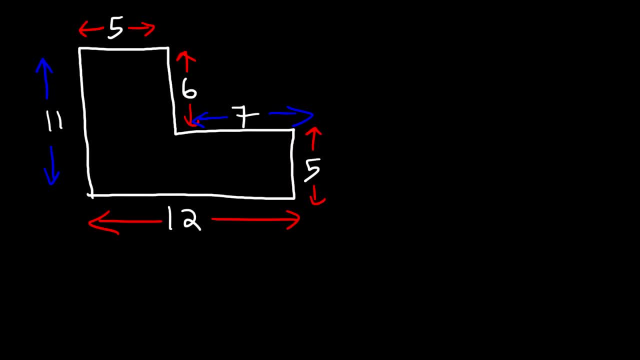 could find the perimeter. We just have to add up all the numbers. So it's going to be 5 plus 6, which is 11, plus 7, that's 18.. 18 plus 12 is 30.. 30 plus 11,, that's 41,. 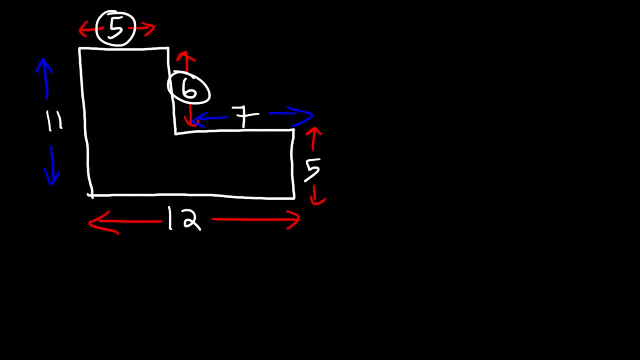 plus 5 is 46.. So, therefore, the perimeter of this figure is 46 units. Now let's find the area of this figure. So let's turn this into two rectangles. So the area of this rectangle is simply length times width, 5 times 6.. So it's 30 square units. 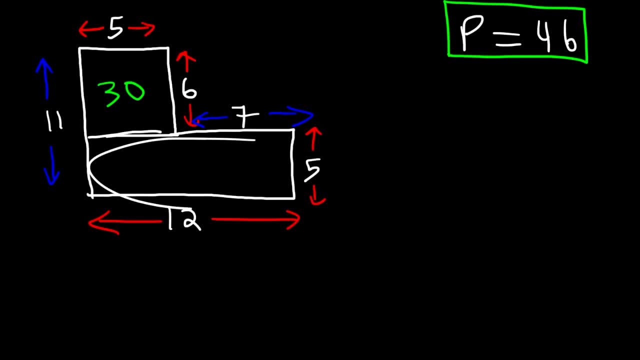 Now the area of the second rectangle is also length times width. So it's 5 times 12, which is 60.. Now to find the total area, we need to add up 30 plus 60.. And 30 plus 60 is 90.. 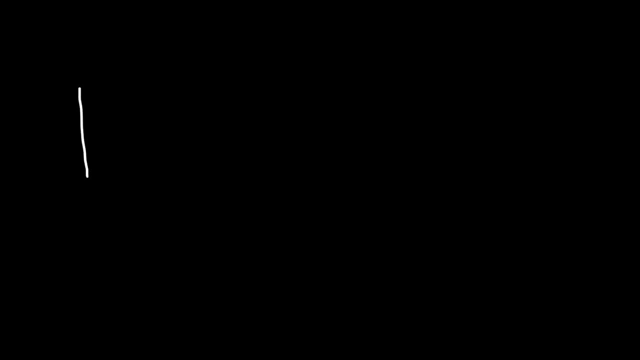 So that's the area of this figure. Now let's work on another example. So let's say: actually let me draw a different figure. Let's say we have a rectangle attached to a semicircle and it measures 5 inches by 6 inches. Find the area and the perimeter. 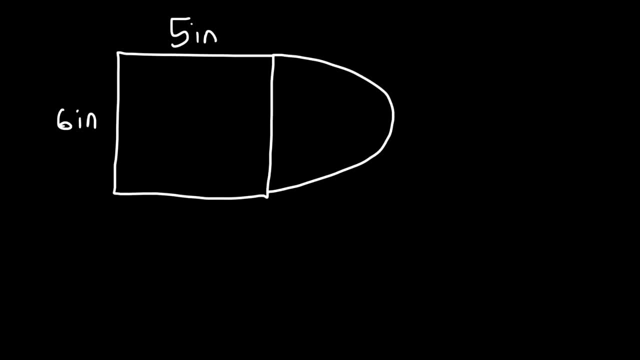 of this figure. So let's start with the area. The area of the rectangle is length times width. So let's start with the area. The area of the rectangle is length times width, Which is going to be 30 square inches. Now, what about the area of a semicircle? Notice: 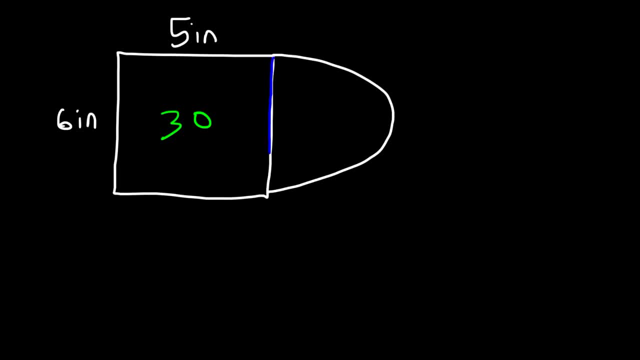 that we have the diameter of the semicircle. The diameter is 6 inches long. So if the diameter is 6, the radius is half of that. Half of 6 is 3.. Now the area of a complete circle is pi r squared The area of a semicircle or half a circle. 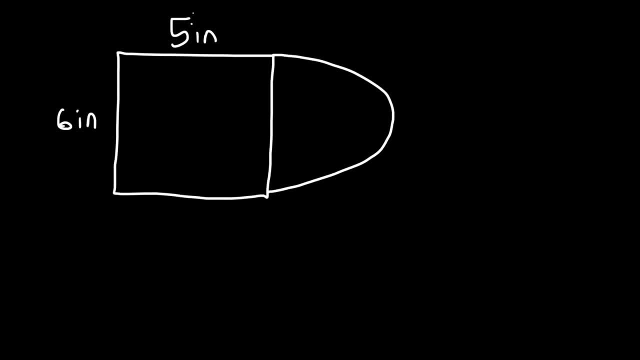 with the area. the area of the rectangle is left times width, which is going to be 30 square inches. now, what about the area of a semicircle? notice that we have the diameters of the semicircle. the diameter is 6 inches long, so if the diameter is 6, 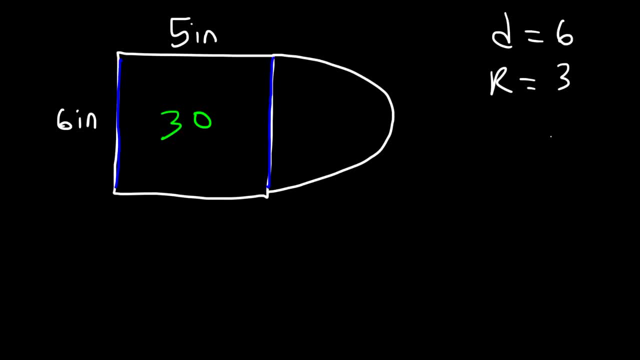 the radius is half of that. half of 6 is 3. now the area of a complete circle is PI R squared. the area of a semicircle or half of circle is one half second, which equals 30ом pi r squared. So it's going to be 1 half pi times 3 squared, Where 3 squared is 9,. 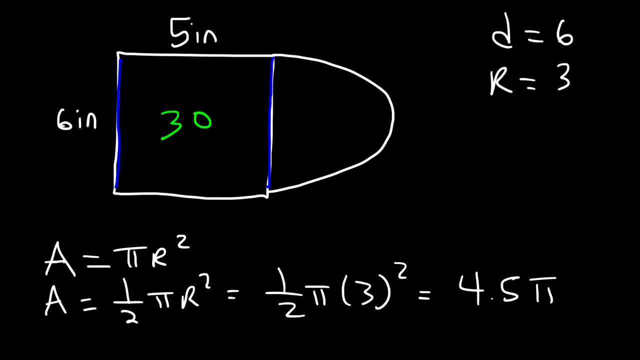 half of 9 is 4.5.. And to get a decimal value let's multiply 4.5 by 3.14.. So this is going to be about 14.1.. So that's the area of the semicircle, So the total area. 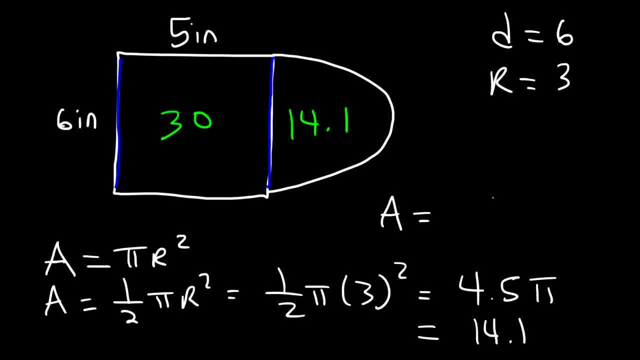 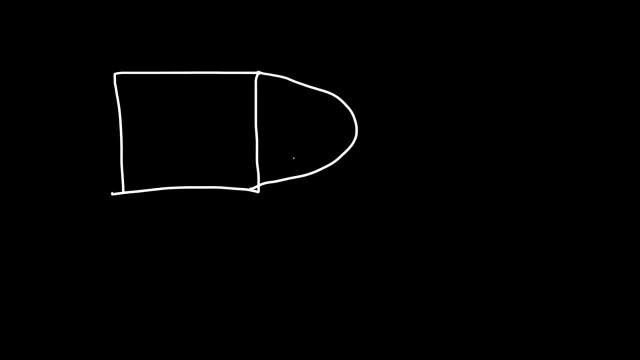 is 30 plus 14.1, or 44.1 square inches. Now I'm going to redraw the same figure and this time we're going to calculate the perimeter. So how can we find the perimeter of this figure? Well, if the top side is 5, the bottom side also has to be 5.. The radius is still. 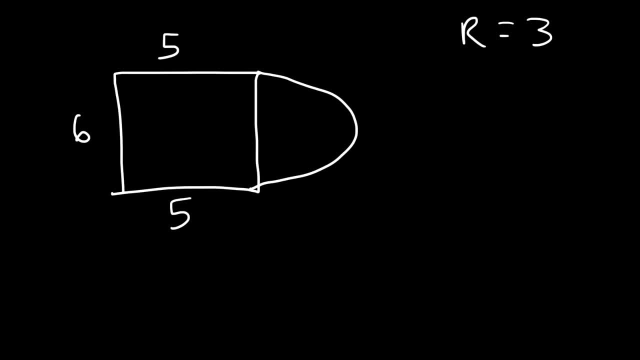 5.5.. So we're going to find the perimeter of this figure. So this time we need to find the circumference of the semicircle. The circumference of a complete circle is 2 pi r. For a semicircle it's half of 2 pi? r, So it's simply pi r. 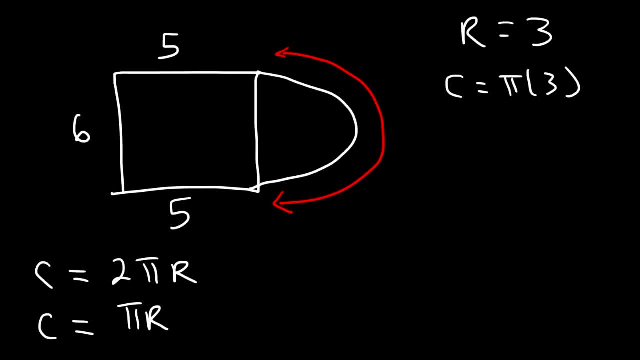 So that's going to be pi times 3.. So 3.114 times 3, that's about 9.42.. That's the circumference of the semicircle. So now to find the perimeter, we just have to add up. 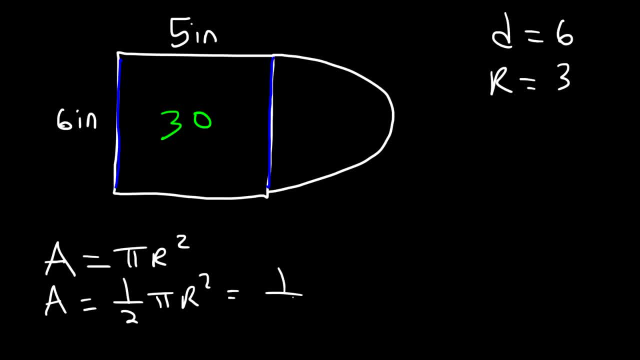 is 1 half pi r squared, So it's going to be 1 half pi times 3 squared. Where 3 squared is 9, half of 9 is 4.5.. And to get a decimal value let's multiply 4.5 by 3.14.. So this: 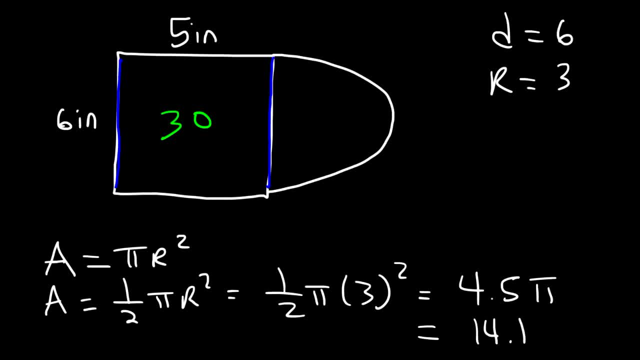 is going to be about 14.1.. So that's the area of the semicircle. So the total area is 30 plus 4.5.. So that's 14.1, or 44.1 square inches. Now I'm going to redraw the same figure And 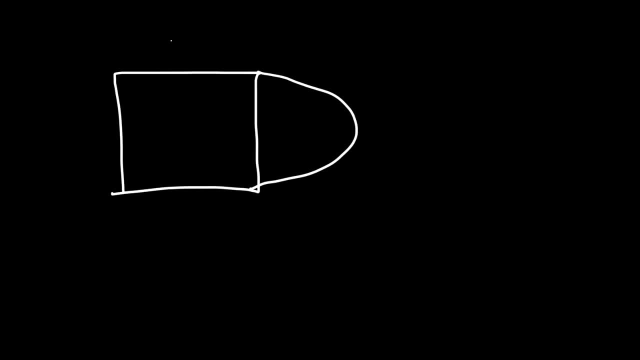 this time we're going to calculate the perimeter. So how can we find the perimeter of this figure? Well, if the top side is 5, the bottom side also has to be 5.. The radius is still 3 units long. 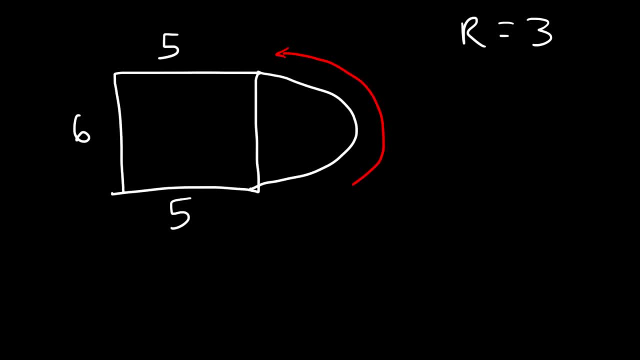 So this time we need to find the circumference of the semicircle. The circumference of a complete circle is 2 pi r. For a semicircle it's half of 2 pi r, So it's simply pi? r. So that's going to be pi times 3.. So 3.114 times 3, that's about 9.42.. That's the circumference. 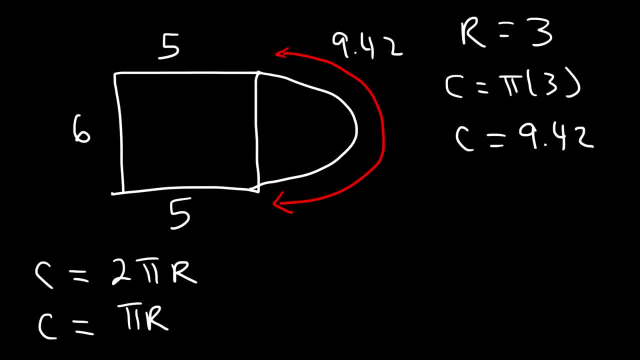 So now to find the perimeter, we just have to add up the four values: 5 plus 5 is 10, plus 6, that's 16. And 16 plus 9.42, that will give us the perimeter, which is 25.42 units. 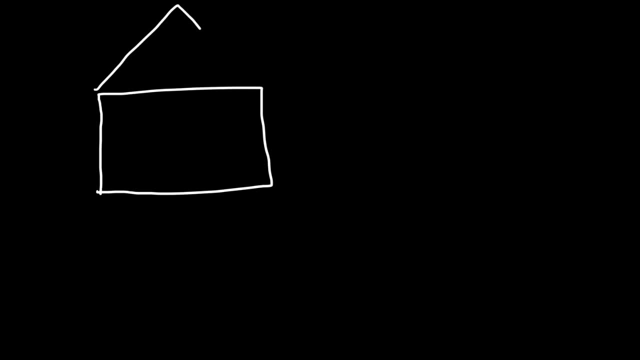 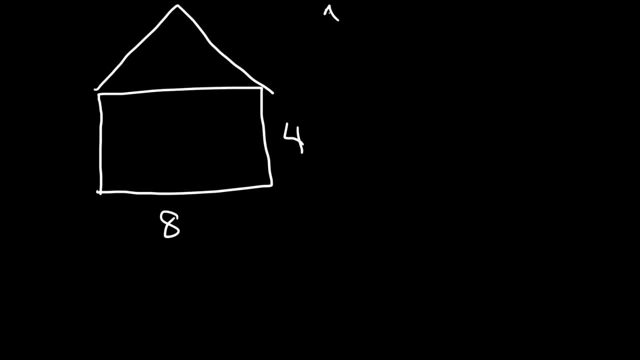 The rectangle is 8 by 4.. The triangle has a height of 4 units And let's say this side is 6, and this is 5.. Let's find the area first. So the area of the rectangle is going to be left times width. 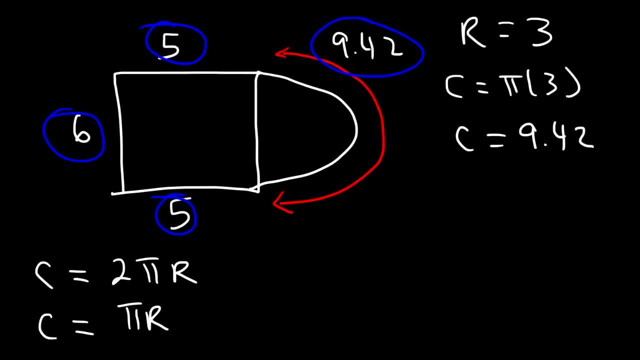 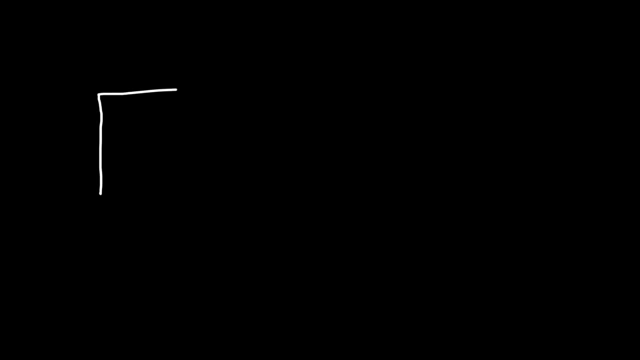 the four values: 5 plus 5 is 10, plus 6,, that's 16.. And 16 plus 9.42, that will give us the perimeter, which is 25.42 units. Let's work on another example. 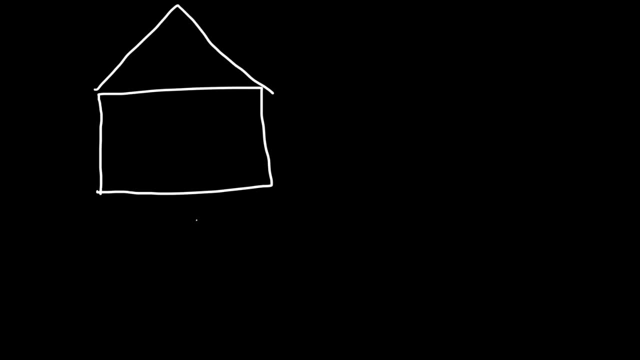 So let's say, if we have a triangle attached to a rectangle, The rectangle is 8 by 4.. The triangle has a height of 4 units And let's say this side is 6 and this is 5.. Let's find the area first. 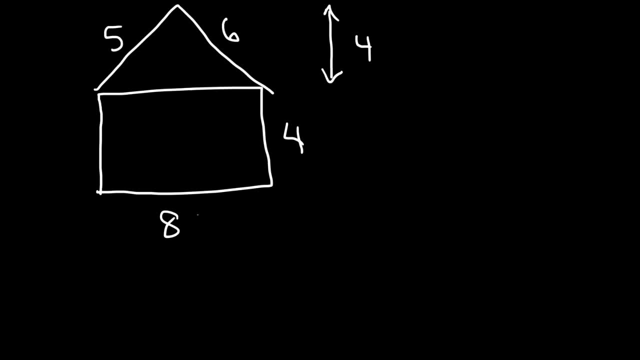 So the area of the rectangle is going to be length times width, So 8 times 4, that's 32.. Now what about the area of the triangle? The area of a triangle is 1 half base times height. So the triangle has a base that's 8 units long and it has a height of 4 units. 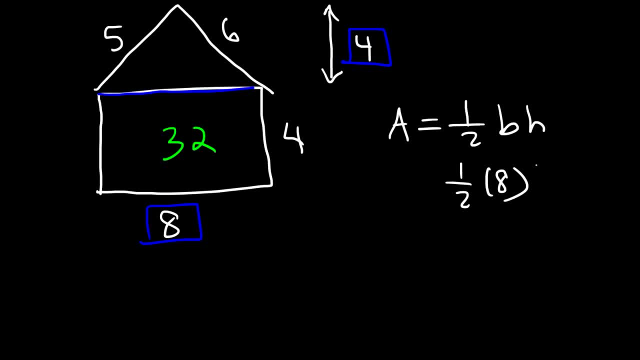 So it's going to be 1 half 8 times 4.. 8 times 4 is 32.. Half of 32 is 16.. So that's the area of the triangle. So now the total area is going to be 16 plus 32.. So it's 48 square units. 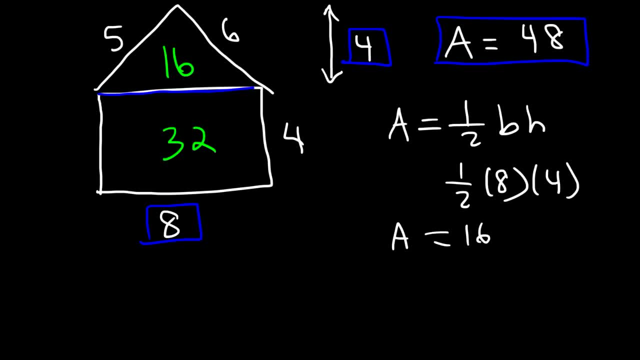 for the entire figure. Now, the last thing we need to do is calculate the perimeter. If this side is 4, this side must be 4.. So, therefore, we'll need to add up all 5 sides, So it's going to be 4 plus 5, plus 6, plus 4.. 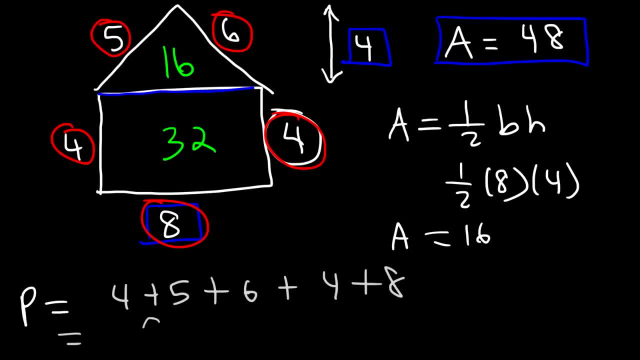 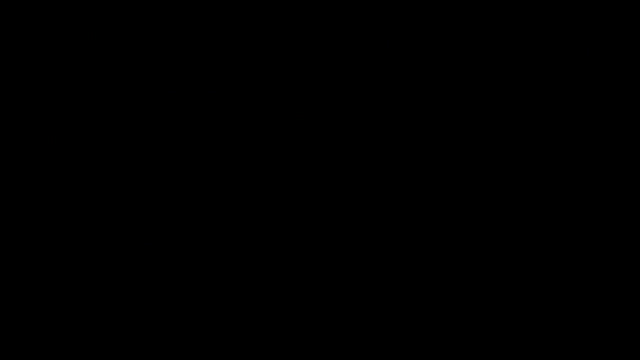 plus 8.. 4 plus 5 is 9.. 6 plus 4 is 10.. 9 plus 10,, that's 19.. And so 19 plus 8 is 27.. So therefore, it's 27 units long. So that's the perimeter of the figure. Now let's move on. 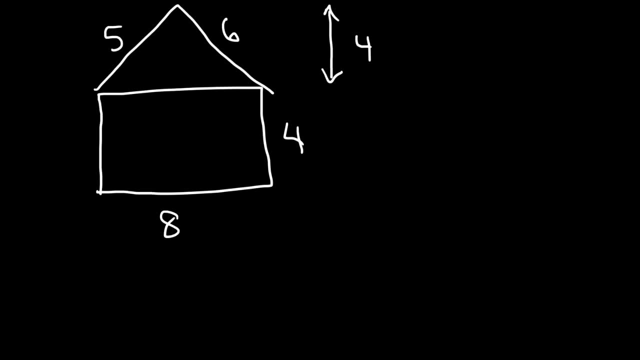 So 8 times 4? That's 32.. Now, what area of the triangle? the area of a triangle is 1 half base times height. so the triangle has a base that's eight units long and it has a height of four units. so it's going to be 1 half 8 times 4. 8 times 4 is 32. half of 32 is 16. so 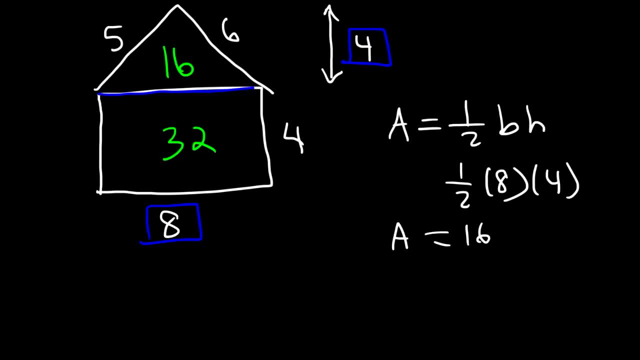 that's the area of the triangle. so now the total area is going to be 16 plus 32, so it's 48 square units for the entire figure. now the last thing we need to do is calculate the perimeter. if this side is for, this side must be for. so 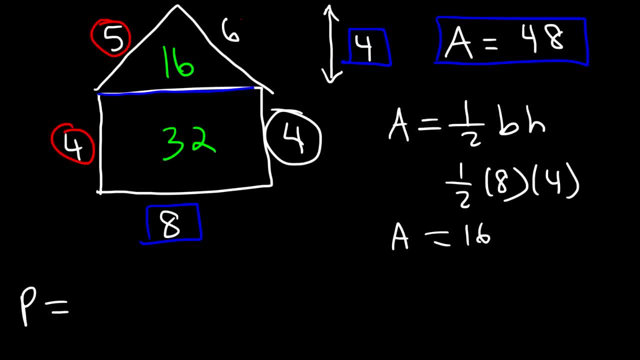 therefore, we need to add up all five sides, so it's going to be four plus five plus six, 6 plus 4 plus 8.. 4 plus 5 is 9.. 6 plus 4 is 10.. 9 plus 10, that's 19.. And so 19 plus 8. 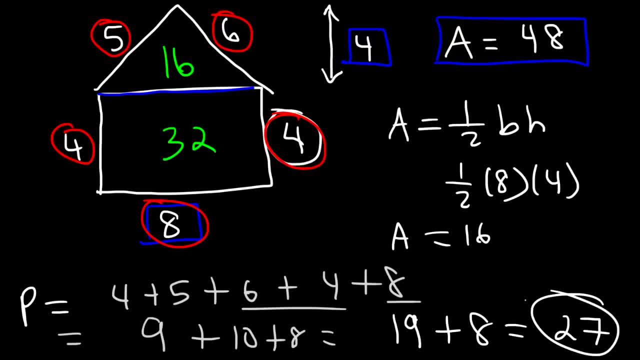 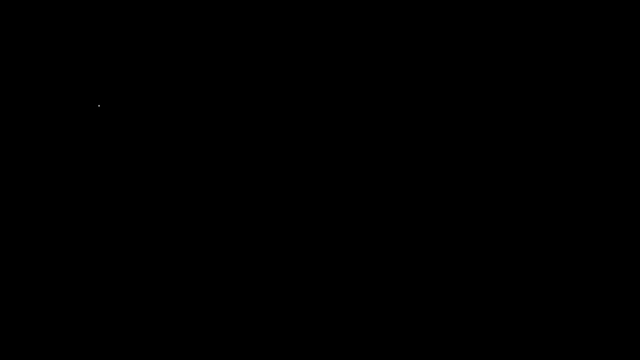 is 27.. So, therefore, it's 27 units long. So that's the perimeter of the figure. Now let's move on to our next example. Let's put a semicircle on top and a triangle on the bottom. So we're going to say this is 7,, this part is 7, and 15,, 12, and 9.. So go. 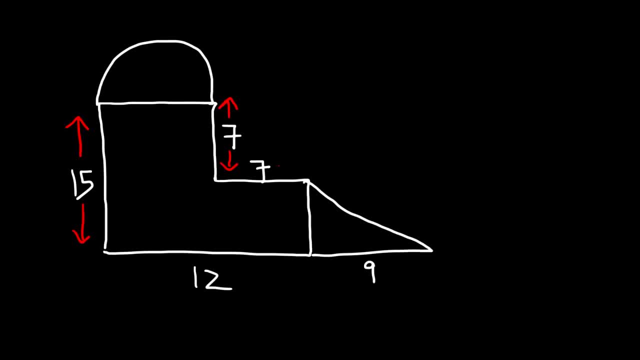 ahead and take a minute, pause the video and find the area and the circumference. I mean not the circumference, but the area and the perimeter of this figure. So let's start with the area. Let's make a line Now. if this side is 7 and this is 15,. 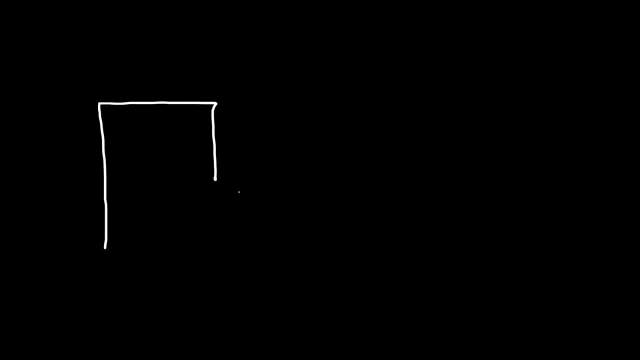 to our next example. Let's put a semicircle on top and a triangle on the bottom. So we're going to say: this is 7,, this part is 7, and 15,, 12, and 9.. So go ahead and take a look. 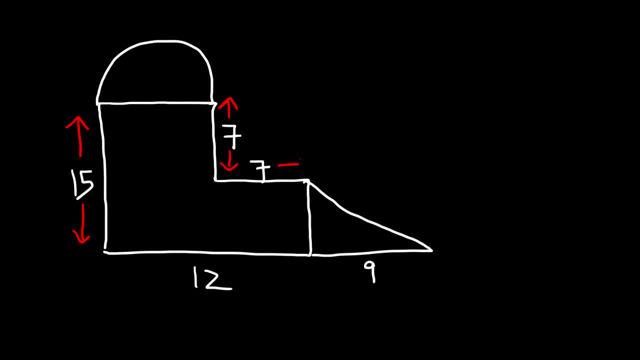 at this. Take a minute, pause the video and find the area and the circumference. I mean not the circumference, but the area and the perimeter of this figure. So let's start with the area. Let's make a line Now. if this side is 7 and this is 15, therefore, 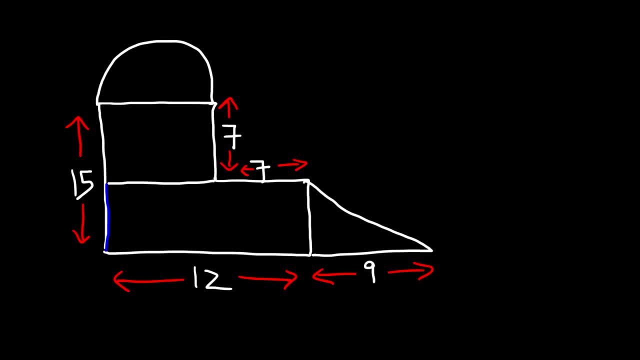 this section has to be 15 minus 7. So it's 8. Since 7 plus 8 adds up to 15.. So now we can find the area of this rectangle. It's going to be length times width, so 12 times. 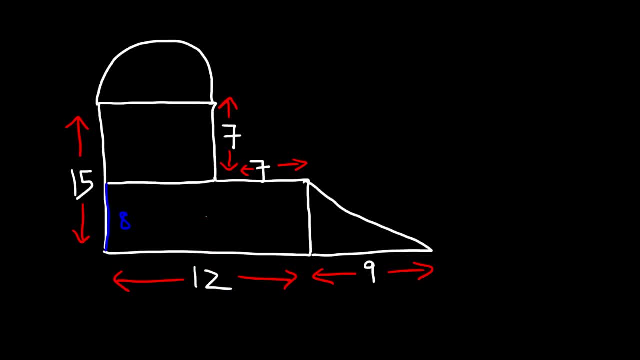 8.. 12 times 8 is 96.. We can also find the area of this rectangle as well. Now we need to know how long the rectangle is. So notice that this side is 12 and this side is 7.. Therefore, this side must be the difference of 12 and 7.. So it's. 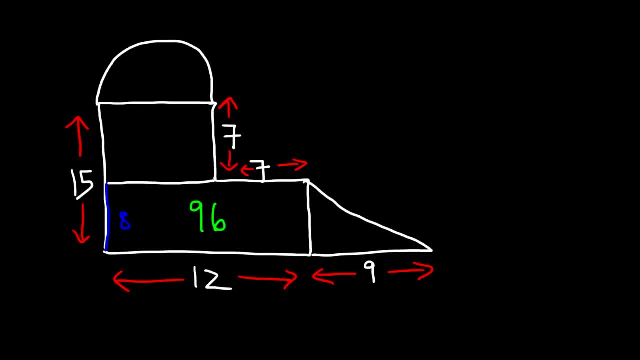 5.. So let's put 5.. So now we can find the area. The area of that rectangle is going to be 5 times 7, which is 35 square units. Now we can find the area of the triangle. It has a height of 8 and a base of 9.. So the area. 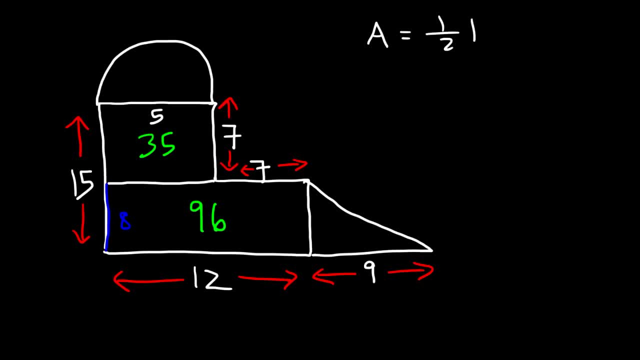 of a triangle is 1 half base times height. So that's 1 half 9 times 8.. Half of 8 is 4.. 4 times 9 is 36.. So the area of the triangle is 36 square units. Now we can focus on the semicircle. 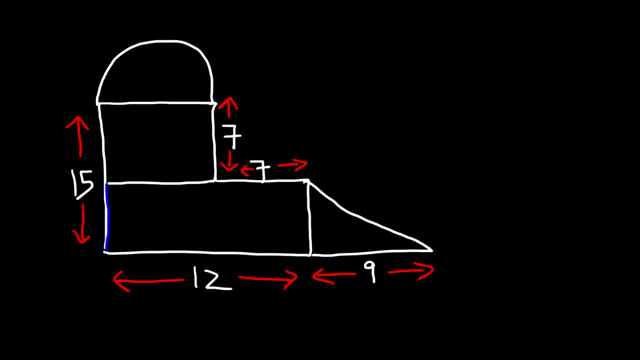 this section has to be 15 minus 7. So it's 8. Since 7 plus 8 adds up to 15.. So now we can find the area of this rectangle. It's going to be length times width, so 12 times. 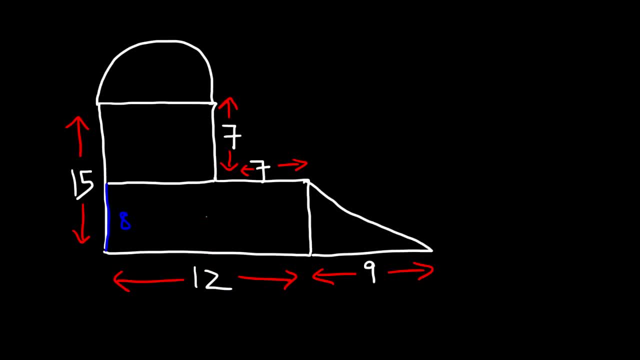 8.. 12 times 8 is 96.. We can also find the area of this rectangle as well. Now we need to know how long the rectangle is. So notice that this side is 12 and this side is 7.. Therefore, this side must be the difference of 12 and 7.. So it's. 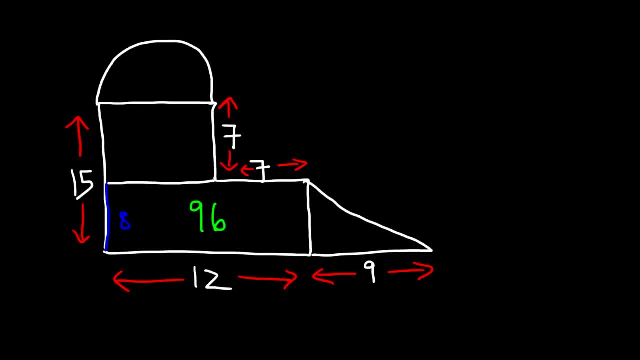 5.. So let's put 5.. So now we can find the area. The area of that rectangle is going to be 5 times 7, which is 35 square units. Now we can find the area of the triangle. It has a height of 8 and a base of 9.. So the area. 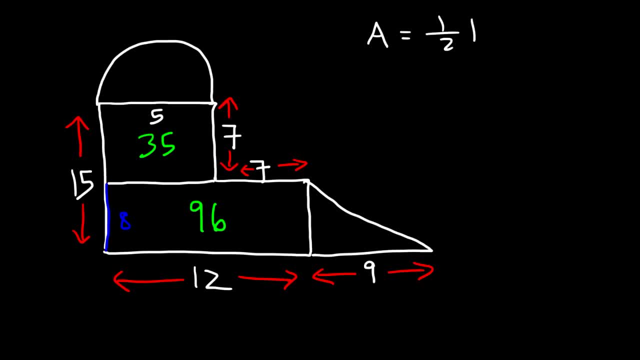 of a triangle is 1 half base times height. So that's 1 half 9 times 8.. Half of 8 is 4.. 4 times 9 is 36.. So the area of the triangle is 36 square units. Now we can focus on the semicircle. 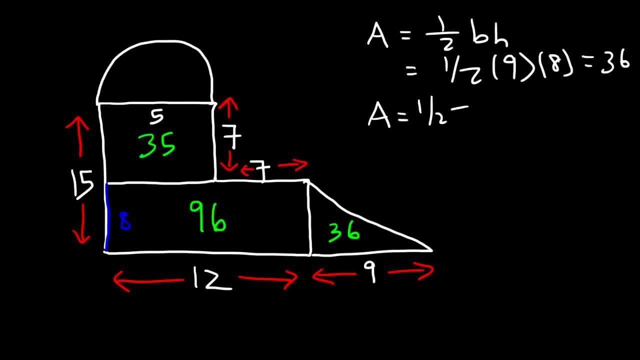 The area of a semicircle is 1 half pi r squared, So we've got to find the radius. If the diameter is 5, the radius is half of 5.. So it's 2.5.. 2.5 squared, that's about. 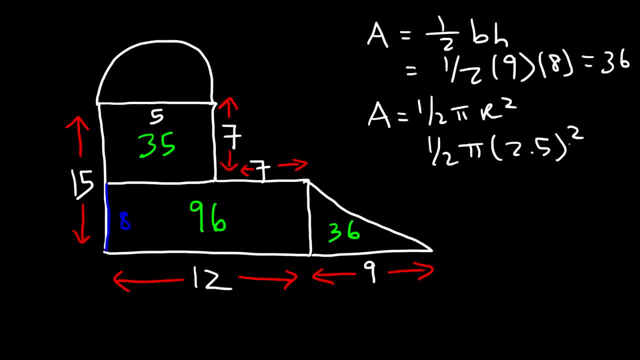 6.25.. If you multiply that by 3.14, that's going to be 6.25.. So we can find the area of the triangle. So we can see we have 36 square units. So that's 5.5 squared. So it's 1 half pi r squared. 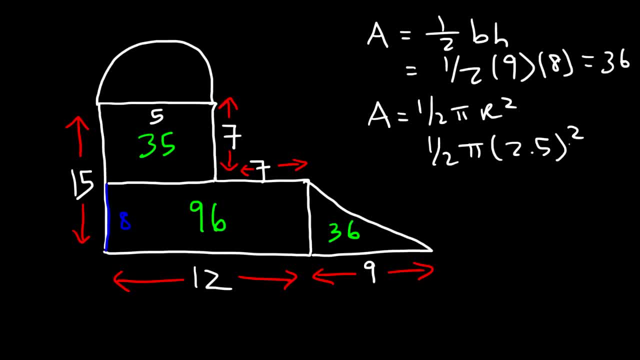 gonna give you about nineteen point six to five and then times it by a half, this will give you an area of nine point eight, one, two, five, which I'm gonna round it and say it's about nine point eight. so let's add up everything ninety six. 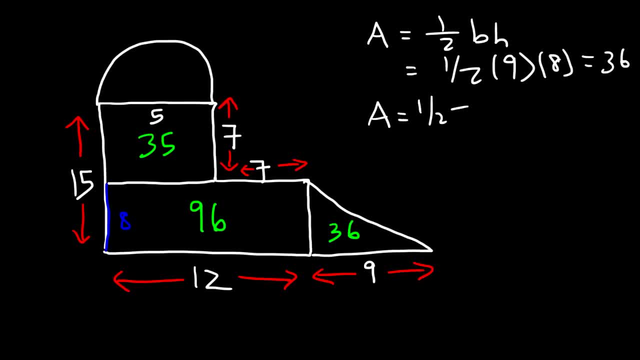 The area of the semicircle is 1 half pi r squared, So we've got to find the radius. If the diameter is 5, the radius is half of 5.. So it's 2.5.. 2.5 squared, that's about. 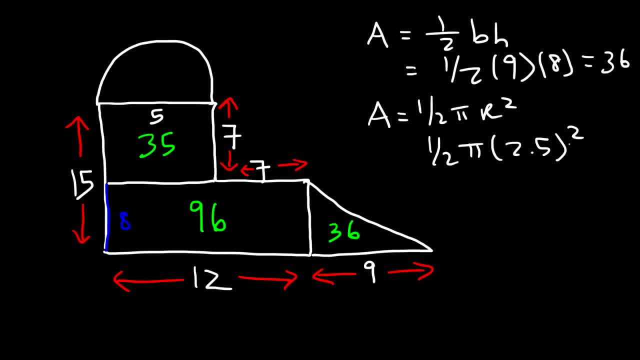 6.25.. If you multiply that by 3.14, that's going to give you about 19.625.. And then times it by a half, this will give you an area of 9.8125, which I'm going to round it and say is about 9.8.. 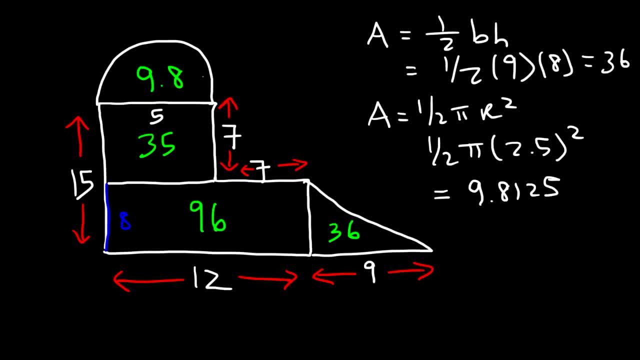 So let's add up everything: 96 plus 35 plus 36 plus 9.8.. That will give us a total area of 176.8.. of the figure, So now we need to find the perimeter. So first let's find the. 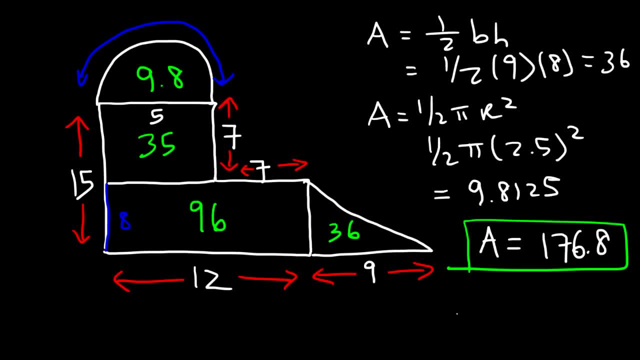 circumference of the semicircle. We know the circumference is half of 2 pi r, or simply pi r. So it's going to be pi times 2.5.. So 2.5 times 3.14 is the circumference. So that's going to be 7.85 units long. Now, the only thing we need to 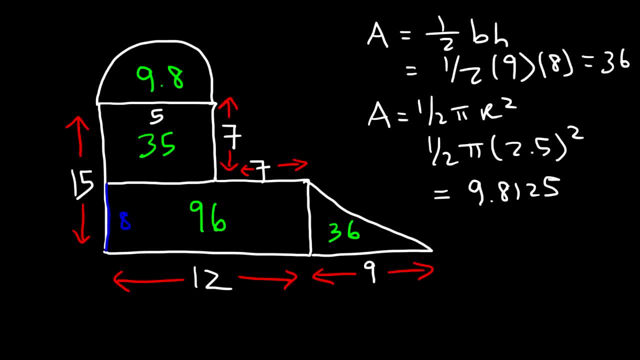 plus thirty five plus thirty six plus nine point eight, that will give us a total area of a hundred seventy six point eight. so that is the area of the figure. so now we need to find the perimeter. so first let's find the circumference of the semicircle. we know the circumference is half of two pi R or. 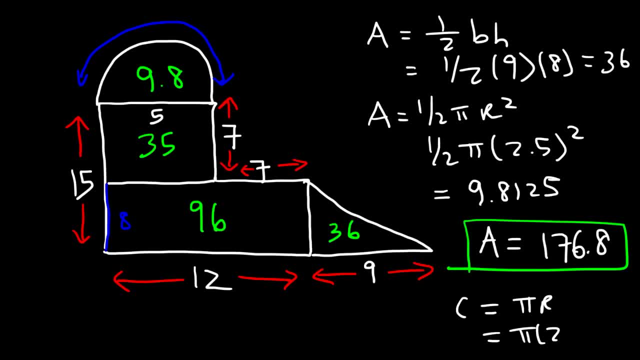 simply pi R, so it's going to be pi times two point five. so two point five is the circumference of the semicircle, and then we need to find the hypotenuse of the right triangle. we have a base of nine, a height of eight, and so to find the hypotenuse we can use the Pythagorean theorem a. 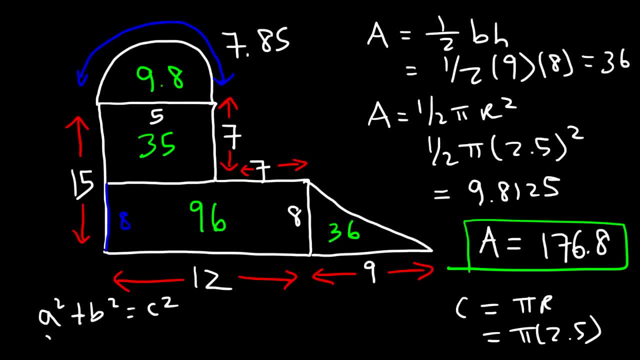 squared plus B squared equals C squared. so nine squared plus eight squared, that's equal to C squared. nine squared is eighty one. eighty-one is the circumference of the semicircle, so that's going to be seven. eight squared is sixty four, and if we add those two numbers that's going to. 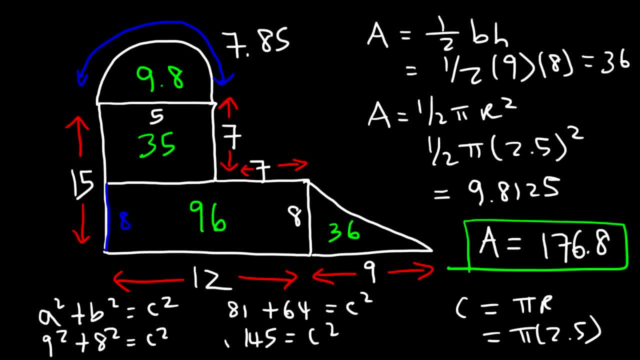 give us a hundred and forty five. so C is the square root of 145, which is about it's twelve point zero four. but we can, we'll write it just like that. so now we need to add up everything to find the perimeter. so we need to add nine, twelve, fifteen, seven, point eight. 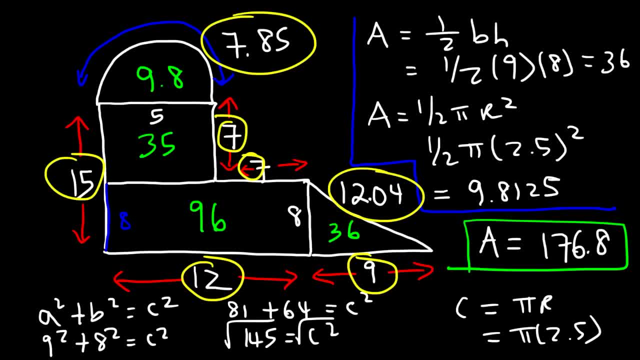 five, seven, seven and twelve point zero four. twelve and nine adds up to 21, and then, once you add 15, that's 36, and then plus seven point eight, five, and then, if you add seven and seven and then twelve point zero four, you should get a. 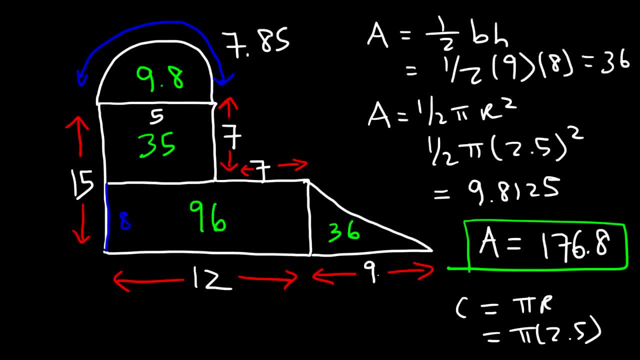 do is find the hypotenuse of the right triangle. We have a base of 9, a height of 8. And so to find the hypotenuse, we can use the Pythagorean theorem: a squared plus b squared equals c squared. So 9 squared plus 8 squared, that's equal to c. 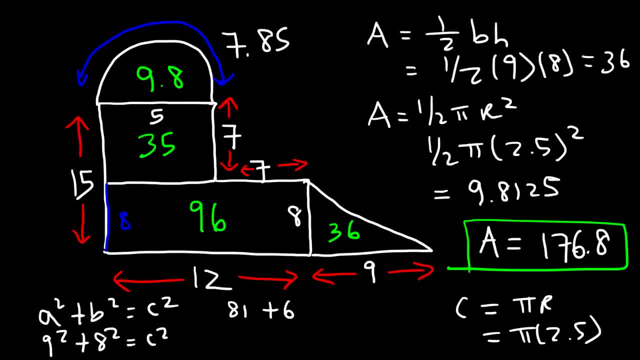 squared, 9 squared is 81,, 8 squared is 64.. And if we add those two numbers we get the circumference of the semicircle. So that's going to be 7.85 units long, And if we add those two numbers that's going to give us 145.. So c is the. 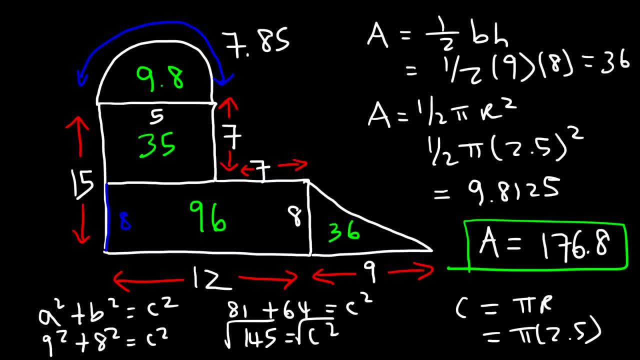 square root of 145, which is about it's 12.04,. but we can, we'll write it just like that. So now we need to add up everything to find the perimeter. So we need to add 9,, 12,, 15,, 7.85,, 7,, 7, and 12.04.. 12 and 9 adds up to 21.. And then 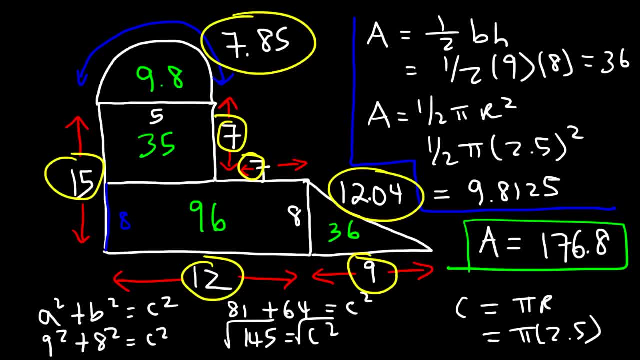 once you add 15,, that's 36, and then plus 7.85.. And then, if you add 7 and 7, and then 12.04, you should be able to find any ungefähr. So we're going to add our. 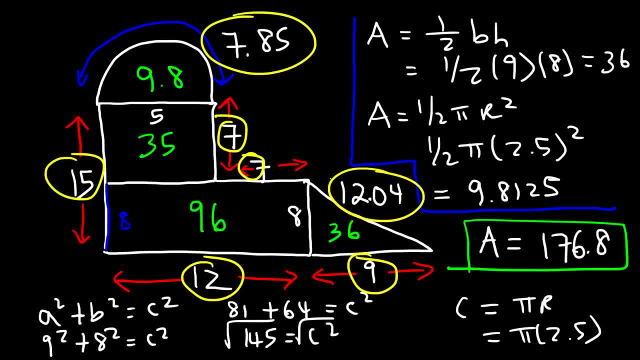 circumference up to 21, plus 7.85. And then, if you add 6, and then plus 7.85,, we get 12.04 units long. So this is going to be 11.04 units long, So we're. 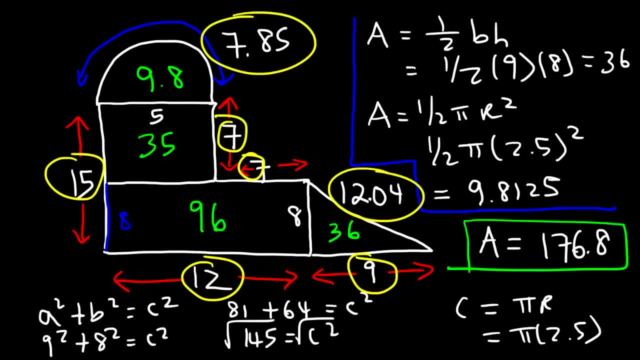 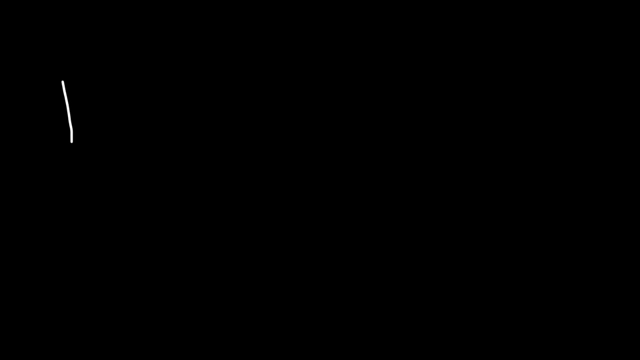 get a perimeter of 69.89.. At least that's what I got. I'm going to double check my numbers just to make sure I typed in everything correctly, But that should be it: 69.89.. So now you know how to find the area and a perimeter of irregular figures. So just to review, here's some formulas. 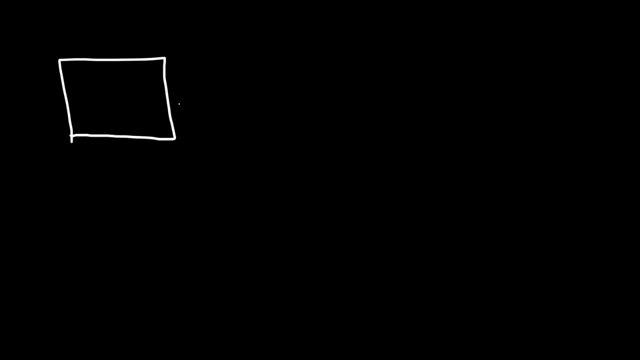 you need to know. Let's say, if you have a rectangle, The area of a rectangle is length times width. The perimeter is simply the sum of all four sides: It's 2L plus 2W. Next, if you have a triangle, the area of a triangle is base times height. 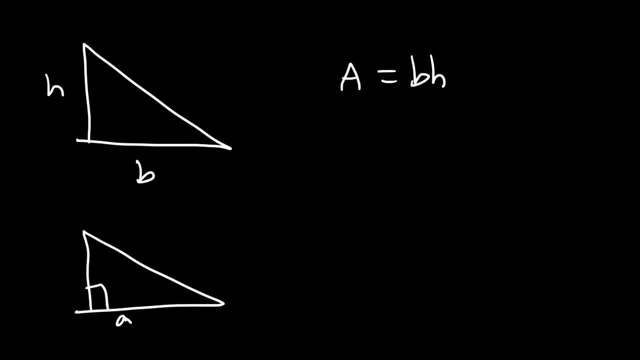 And if you have a right triangle, if you need to find the missing side, you can use the Pythagorean Theorem, And let's not forget to put the 1 half in front of the base times height for a triangle. Now, the last other thing that we've considered is a circle, The 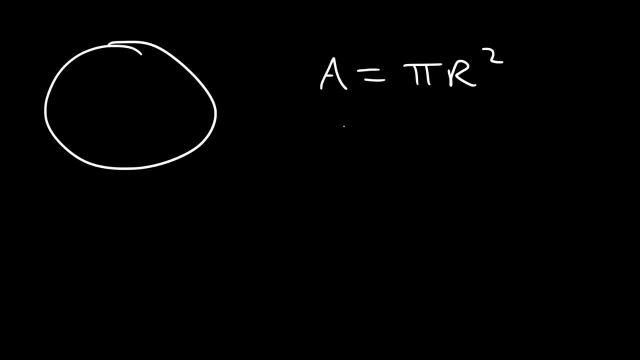 area of a circle is pi r squared and its circumference is 2pi. And keep in mind the diameter is 2r And pi, if you round it, is 3.14.. Now there are some other numbers after the 4, but in this example we just kept it simple and used 3.14.. For a semicircle, everything. 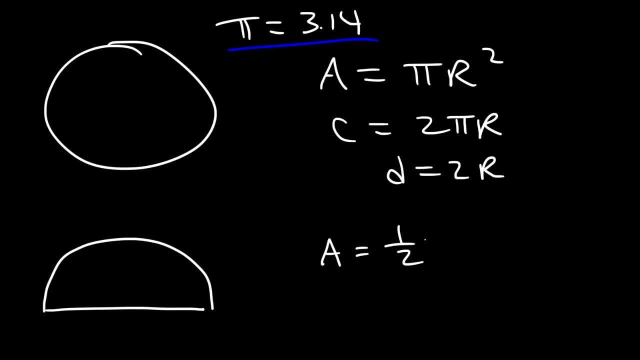 is 1 half, The area is 1 half pi r squared And the circumference is just pi r, But the diameter is still 2r. So this is not going to change. So that's just a recap. So that's just a recap of some of the formulas that we've used in this video. So make sure.